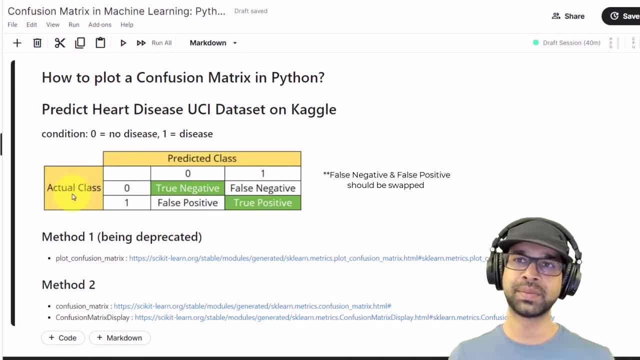 matrix. so if you look at this confusion, matrix, it's going to be looking something like this, where we have the actual class on one side- zero- and one predicted class- zero- and one now anything that is zero. that is actually, it was zero and we predicted zero. it's going to be true, negative. 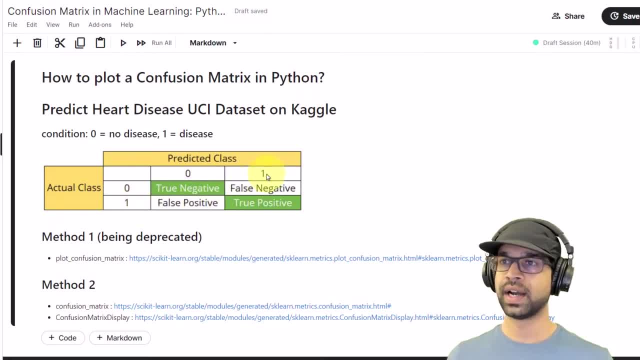 and this is the good thing. similarly, if it's one and we predicted one, it's going to be the true positive, apart from that, any other condition. so if it is zero and we predicted one, it's going to be false negative. and here it was actually one and we. 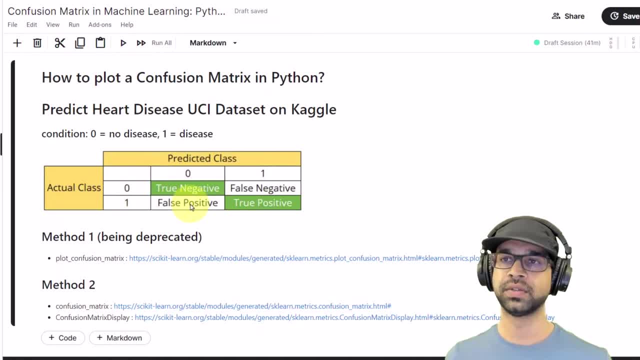 predicted zero, then it's going to be a false positive, and so this way, this confusion matrix will be built and you'll be able to interpret a lot of things on top of this. in this video, we're just going to focus how to plot this confusion matrix. i'm going to make another video on the. 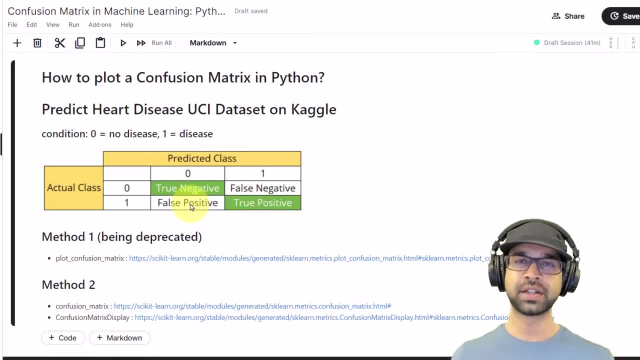 interpretation of it, so do watch out for that also. i've made another video on how to do the same thing on excel. i'll place the link somewhere here or in the description section below and you'll be able to get a more visual way of creating the same matrix. the first method is: 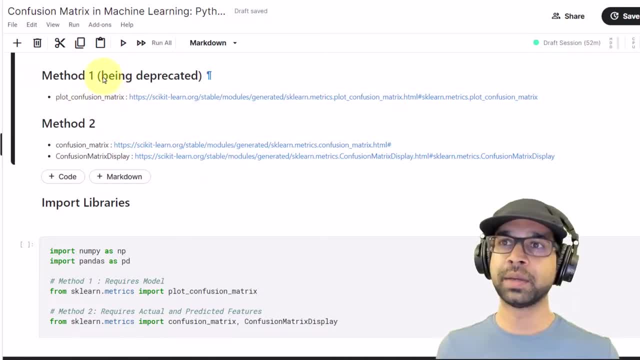 going to be plot confusion, matrix. now this is going to be deprecated. nonetheless, i'm just going to still show it to you how it works, and then i'm going to show you the method that you should implement within your own code. we'll begin by importing the libraries. now we're going to import. 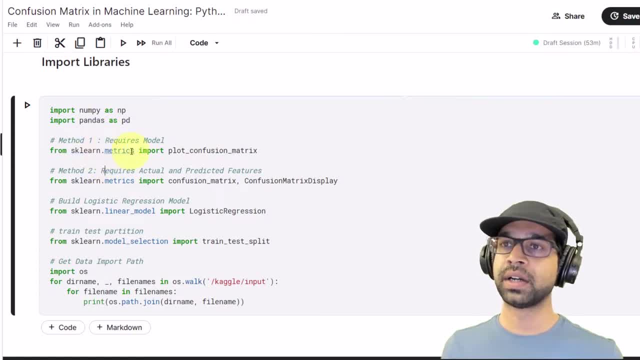 numpy and pandas. then we are going to take escalar matrix plot, confusion matrix- now remember, this is the deprecated one. however, within the same matrix library we have confusion matrix and confusion matrix display. these are the two that we're going to be using in the second method. then we're going to be using the logistic regression model for 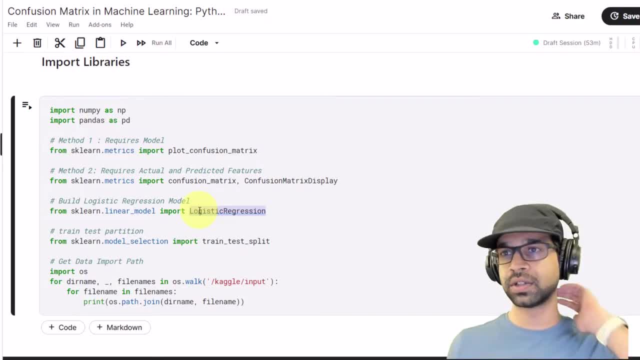 doing a sample model and then making predictions out of it, and so this is going to help us just create the confusion mate. also, we're going to do the trend test partition using the model selection train test split, and we're going to create the confusion matrix on the test data. that means 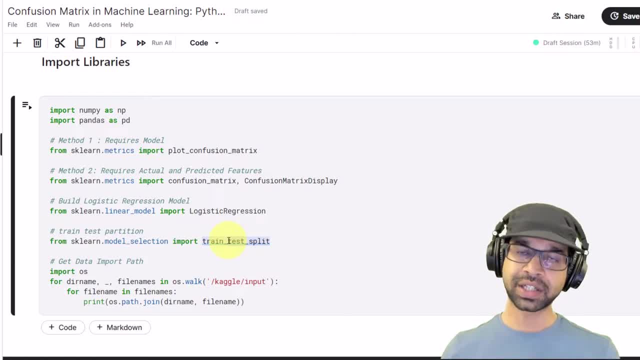 we're going to build the model, make predictions and, on the test, data is where we'll compute the confusion matrix. now, this one will just give us the path of where this data set is present on kaggle. yes, now, if you want to use this and run this code, along with me, you. 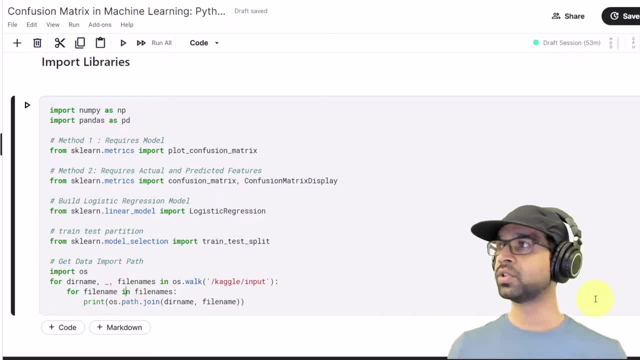 can click on this kaggle link. click on the edit button, which is going to be on the top right corner here, and then you can follow along with me with this particular code. for that you should have a kaggle account, of course. let's run the code to import the libraries. next we're going to begin by 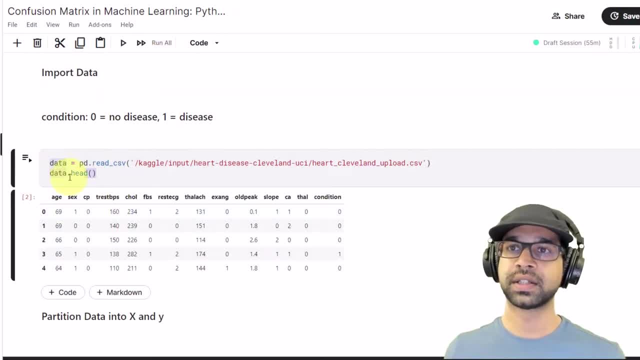 going to run the code to import the data and, if i run this, and this is just the top five rows of this data, so you'll have age, sex, cp and rest of the features, along with condition. now, this is something that we are modeling against and this is what we'll be creating. the confusion matrix on. 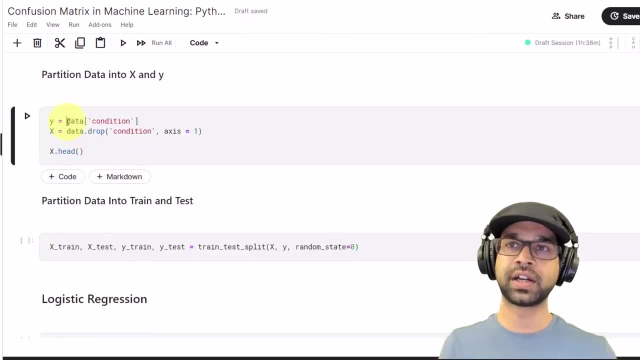 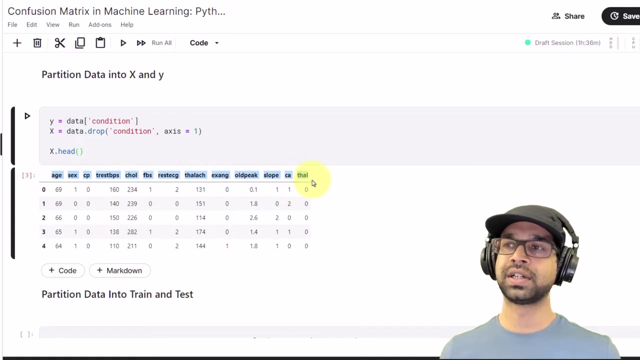 next we'll partition the data into x and y. so we're going to take condition in the y variable and then in the x variable we're going to take everything else apart from condition. so if i run this code we should be able to see all the x variables here. you'll see that condition is. 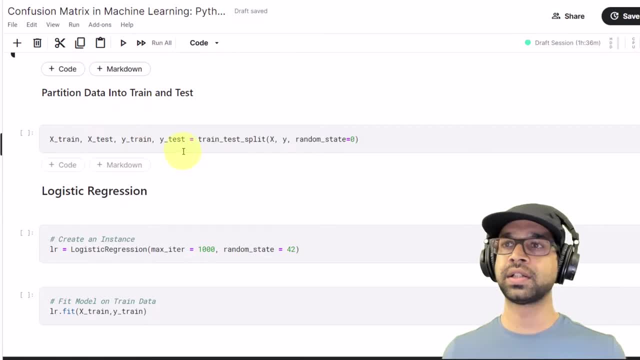 missing here. next, we're going to partition the data into train and test, so we're going to take x and y and we're going to split it into x train, x test, y train, y test. we have used all the default parameters here, except for random state. we just want to keep things consistent, so we have used 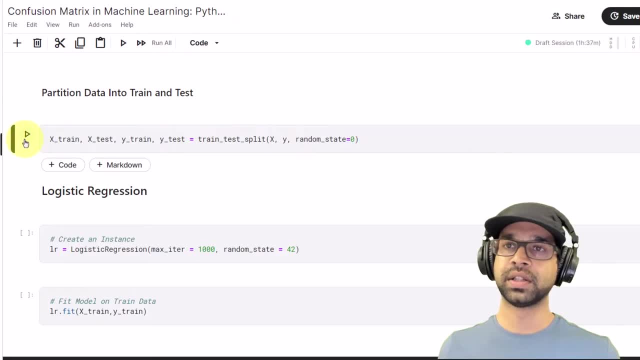 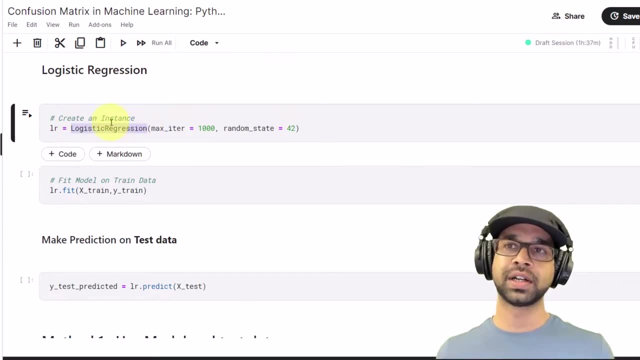 a random state is equal to zero. now let me run this code. now we have two partitions: the train data and the test data. next we'll build the logistic regression model and we're going to create an instance first and i'm going to give. max iteration is equal to 1000. 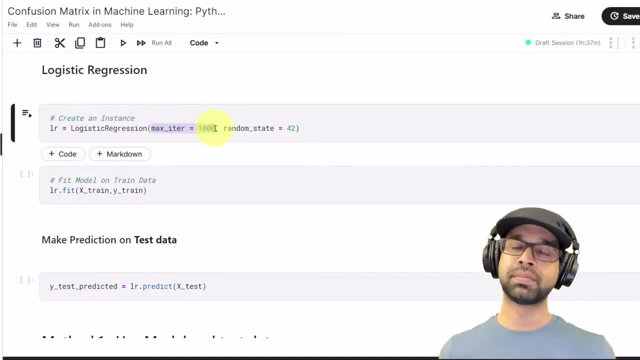 because sometimes it needs to converge and do some good number of iterations before it can get or fit the model- and we want to say random state is equal to 42 here, just to ensure we can replicate these results. so let's run this one first and then fit the model. now the logistic regression model is fit. 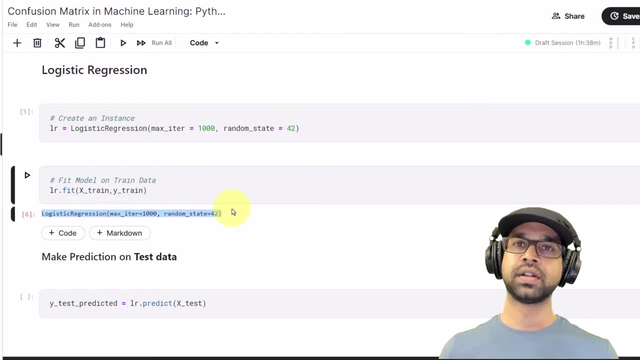 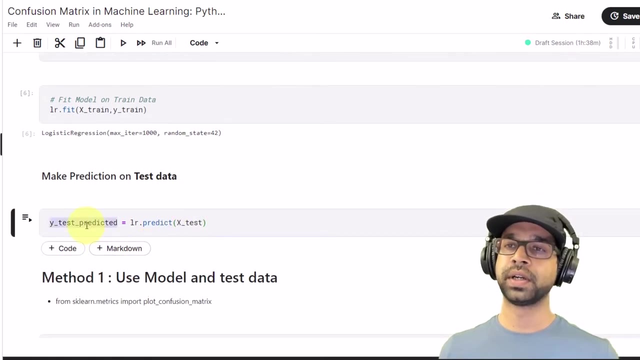 which means we have a model that we can use to predict the condition. so let's predict the condition. i'm going to call the test model predictions as y test predicted and it is equal to lr dot predict x underscore test. i'm going to run this one and what this will do is it will print all the predictions for this particular 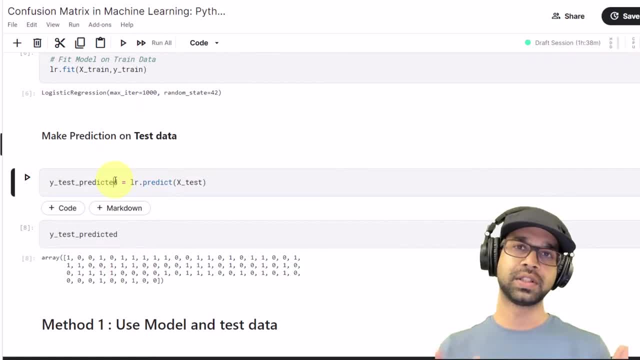 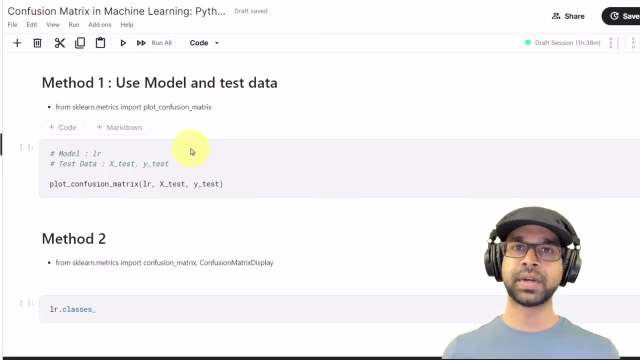 data set, and now we have both the classes, which is the actual classes, and the predicted classes, which is what we will be requiring to build the confusion matrix. let's start with method one. in method one, we're going to require the model. remember, we require the model in this method. 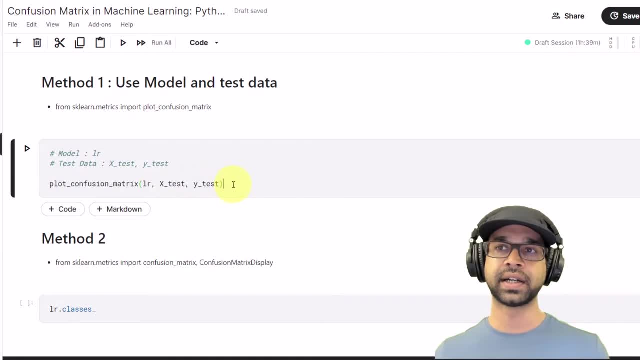 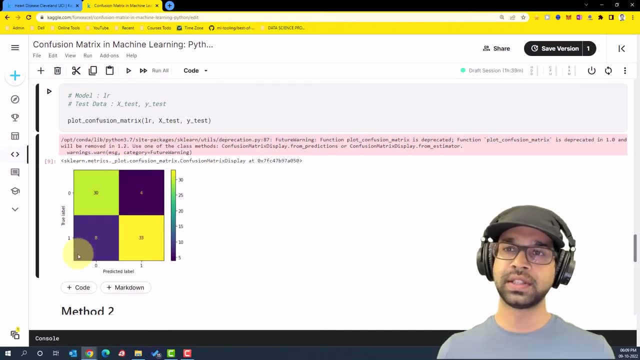 one and along with it that x and y test data, which is this one. now i'm going to plot the confusion matrix with the first method and notice you will see that confusion matrix getting plotted. however, it's going to show a future warning and it says function plot. confusion matrix is deprecated in 1.0. 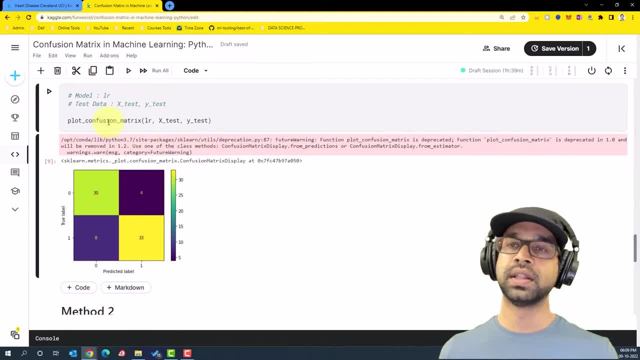 and will be removed in 1.2, which means this function or this method is going to be deleted in the future, which is why we will use the method method in the future, which means this function or this method is going to be deleted in the future, which is why we will 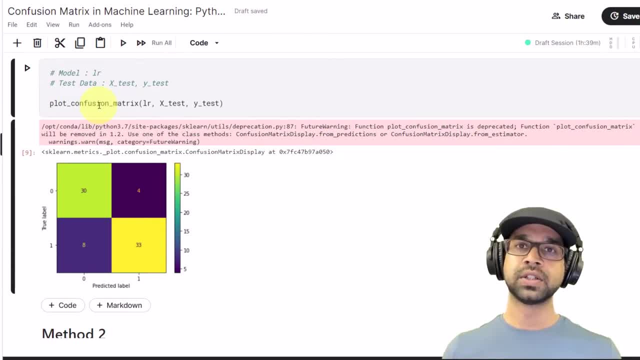 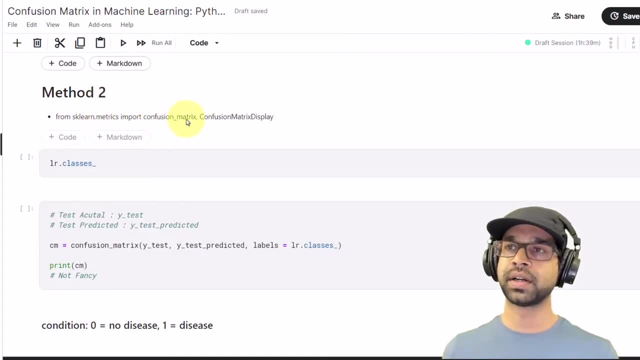 be requiring another way to plot the confusion matrix. so let's look at what the method 2 is. in the method 2 we are going to be requiring two things: one, the confusion matrix and then confusion matrix display. what escalon has done is basically they have divided the confusion matrix into two parts. 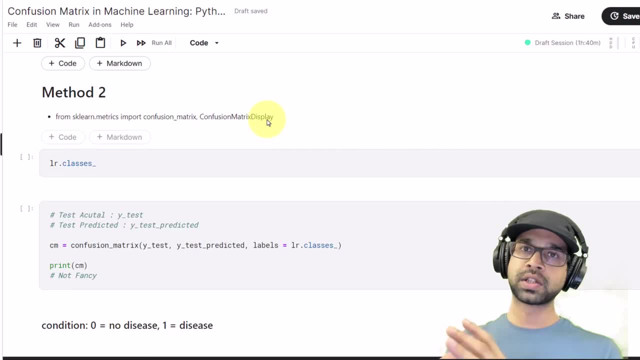 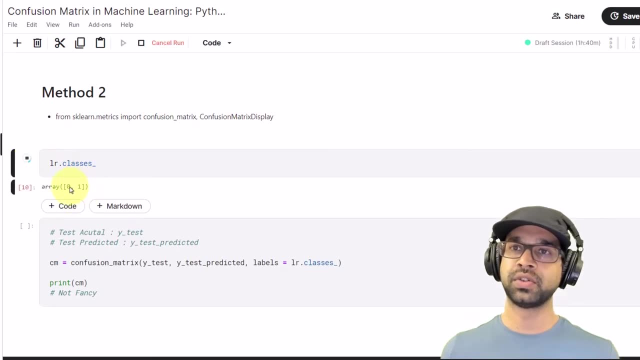 one which actually create, calculates a number, and one which plots it or shows it on a chart. so let's do both of them step by step. first of all, let's look at what are the classes within lr. now, if you look at the regression and you say dot classes, you will see that it will give you an array. 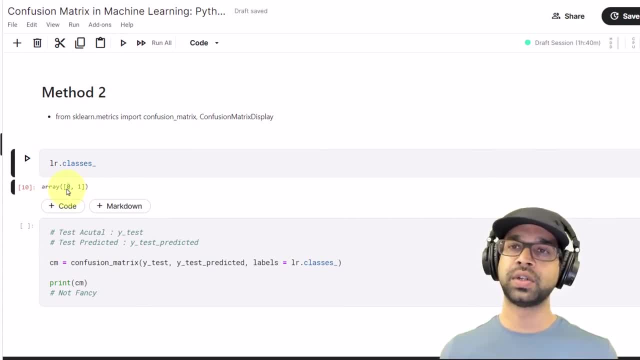 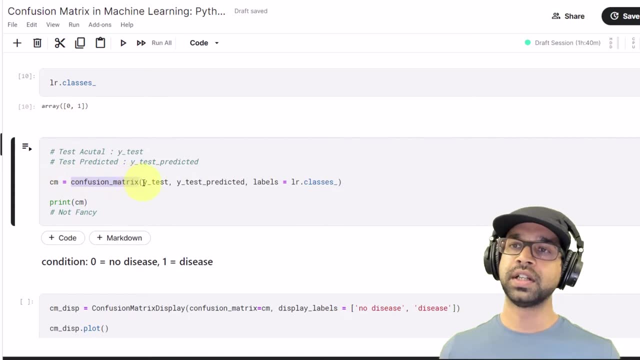 which is zero, and one zero, the condition is no disease, one the condition is a disease. and so, for this particular example, we are going to use the confusion matrix. in the confusion matrix, unlike the method one, we'll require the y test and the y test predicted. we also need to give the 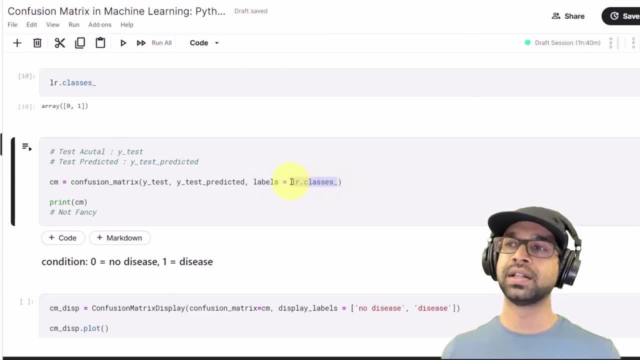 labels. right now, we're just going to give the labels that the logistic regression model has with it. however, we can choose to put any other label. we can choose to put any other label. we can choose to put any other label labels within this space. so let's run this one and see what we get now if we run this. 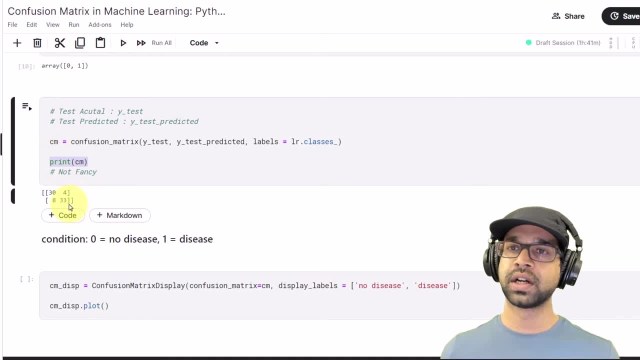 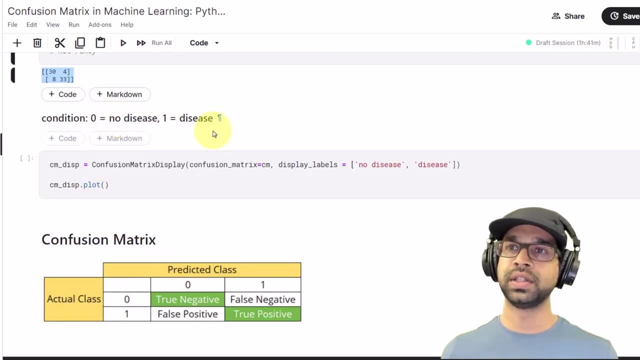 method, you will see that we are getting this confusion matrix. however, it's only giving us the numbers, but it's not that fancy, which is why we require the next function or method, which is going to be confusion matrix display. remember, zero is equal to no disease, one is equal to disease, and so 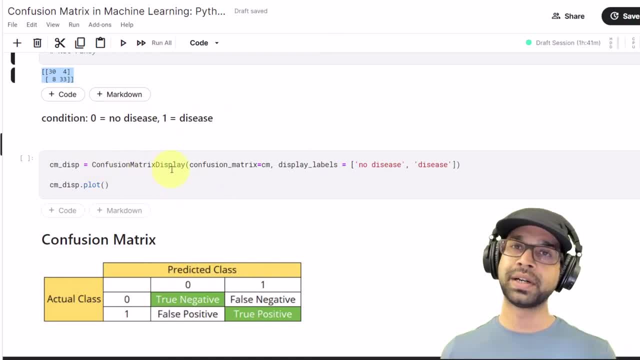 this time we're going to give all the parameters that the confusion matrix display requires, but change the classes a little bit just to ensure that this, the display, looks a lot better. so the confusion matrix display takes the confusion matrix as input. note that we have used this. 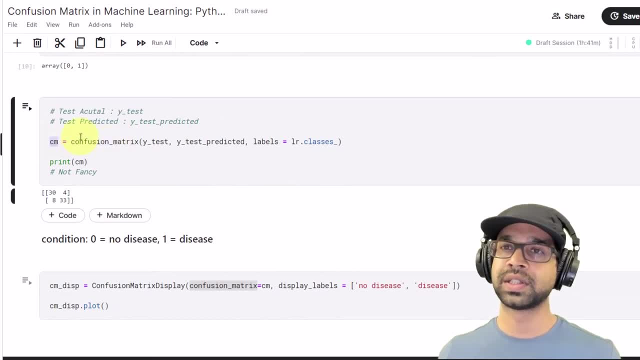 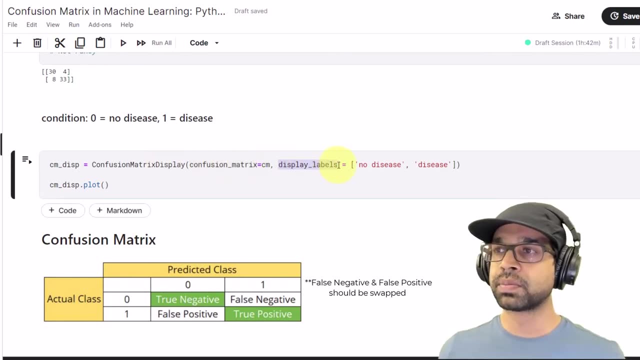 confusion matrix to get it into a variable called cm, and now we are giving this as an argument to the confusion matrix display. next, the display labels is something that we can change here, and so i've decided to go with these. no disease and disease. and note: it should be in the order. 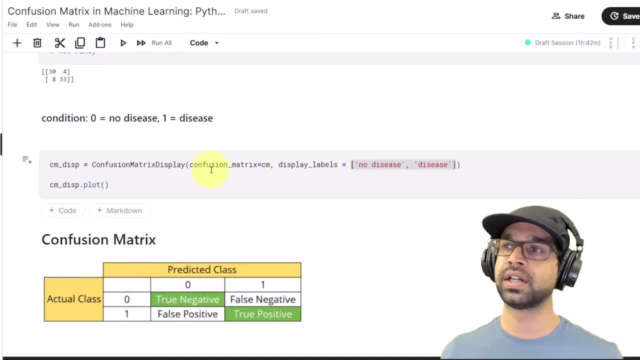 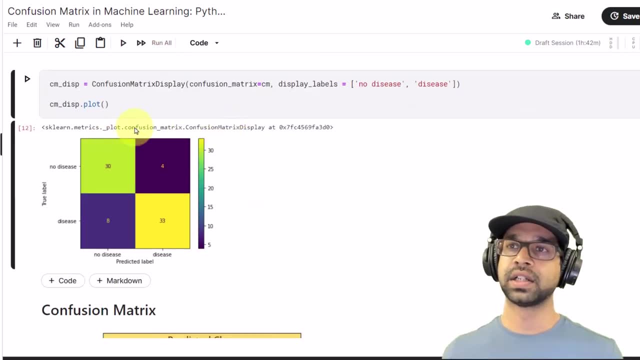 of how you are seeing the lr dot classes here, right? so that is why no disease, and disease is what i have chosen to go with. and now i can finally run this and it should give you the escalon plot confusion matrix notice: we take this into the variable and then we say cm. 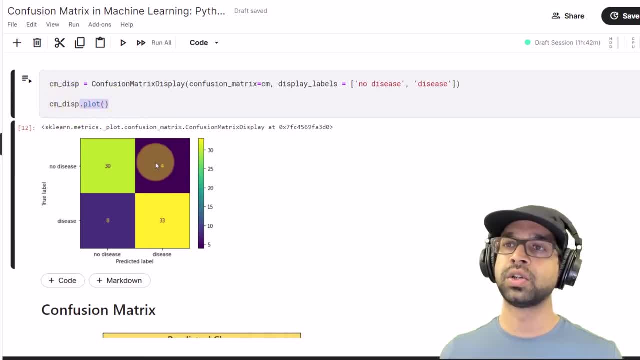 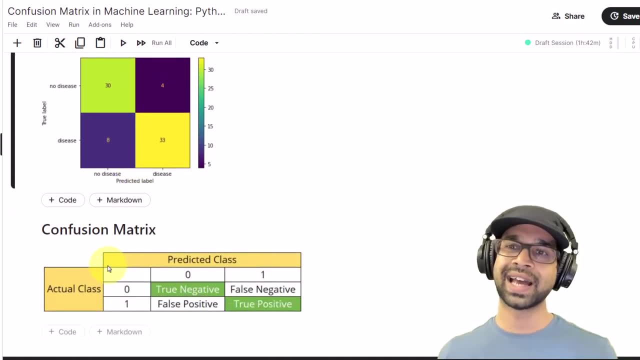 display, that is, confusion matrix display. dot plot to plot the confusion matrix. just to give you a refresher about what this means: confusion matrix has the actual classes, that is, the labels on one side, predicted labels or predicted classes on this side. so this one here is called: 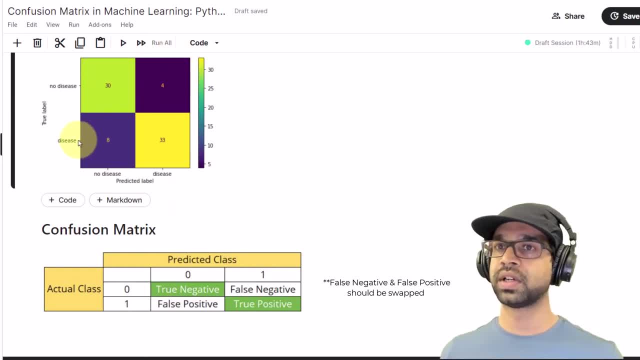 the true negative. this number is false positive, this one is called the false positive and this is called the true positive. initially, you want to begin with looking at the true positive, because that's the matter of focus for this particular case and for your context might be different. 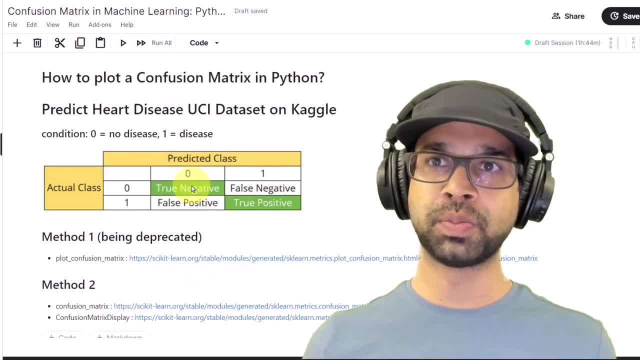 that's all i have for confusion matrix, guys. so now that you know how to plot a confusion matrix using confusion matrix in confusion matrix display, you have to do one thing: first you have to load a number of positive and positive cases, and then you have to count the number of positive cases and then you